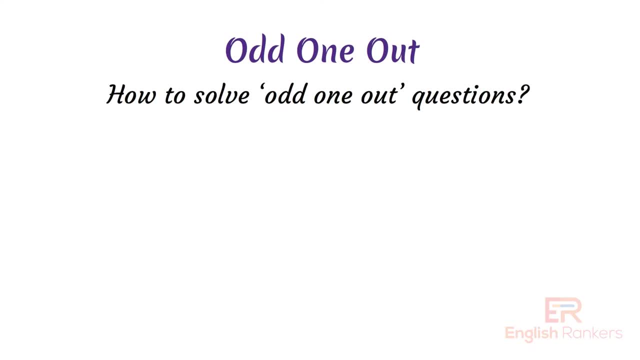 how to solve odd one out questions. there are no specific rules for this. each time you will be given different types of problems. you should be logical and intelligent for finding the answer. though there are no specific rules, you can follow below steps. these can help you to some extent. read all the options. 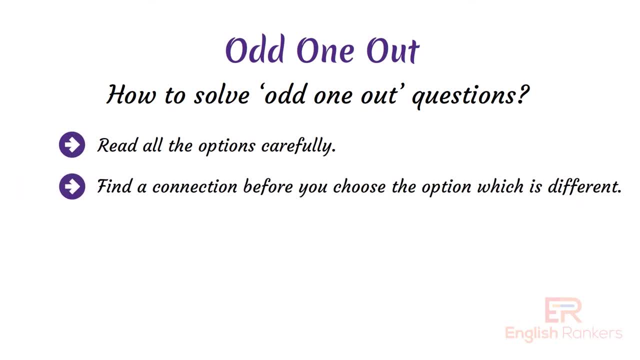 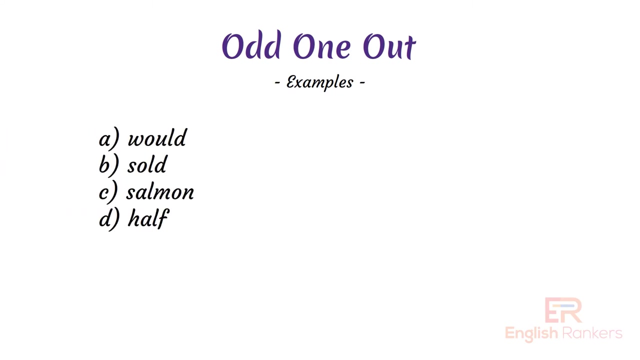 carefully find a connection before you choose the option which is different. if you don't understand an option in the growth, it may be connected to the other options. don't choose an option because you don't understand it. find a connection first. check your answers carefully. when you finish, look a few more examples. a would be sold. C salmon. 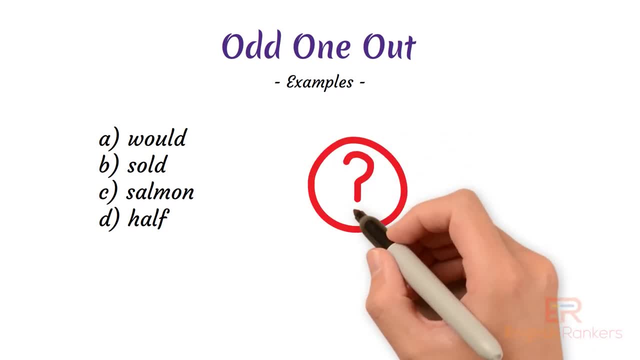 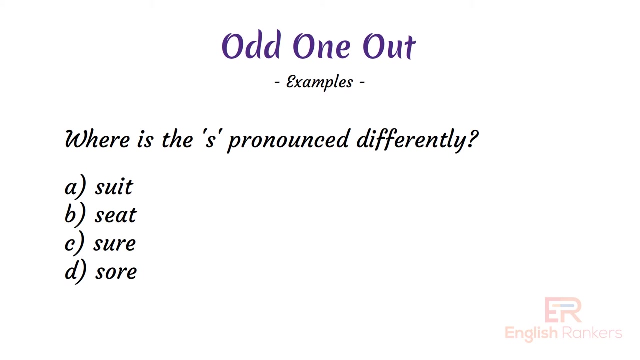 D half. can you tell which one is odd one out and why? you can tell which one is odd one out and why? answer is sold, as L is not silent in sold. next question: can you tell me where is the s pronounced differently? answer is C. sure, here s sounds as such ensure, and in rest of option it is s suit. 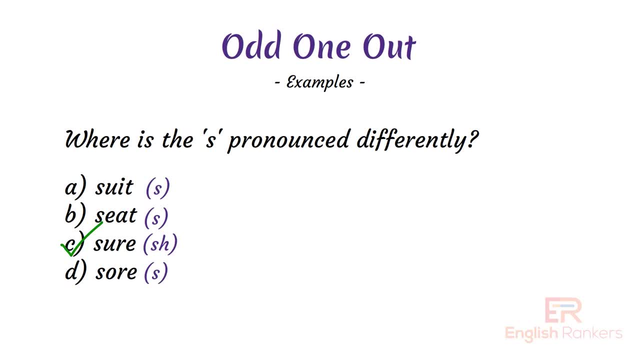 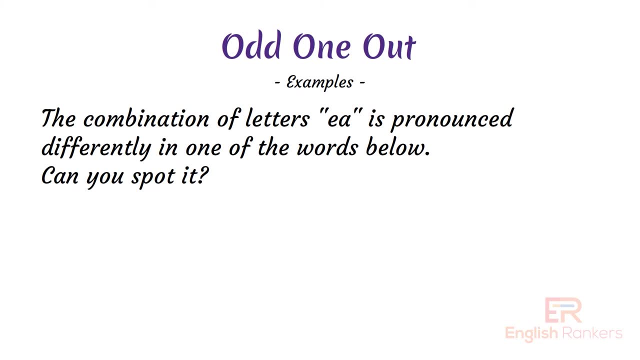 here s comes with a different pronunciation, such as a solid letter, the s is pronounced differently. another way you can explain this is by mixing these two: sau소 outlet of sounds C. so next example: the combination of letters EA is pronounced differently in one of the words below. can you spot it? what will be? 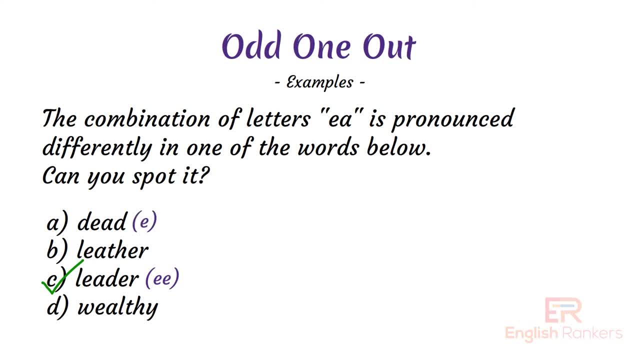 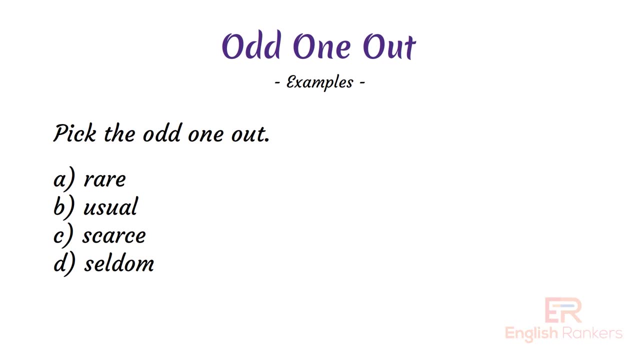 the answer? answer is options. the leader in leader, double E. sound is coming in Leather Wealthy. Pick the odd one out: A- Rare, B- Usual, C Scars, D- Seldom. The answer is B- Usual. Rare Scars Seldom are synonyms of each other, which means uncommon or unusual.